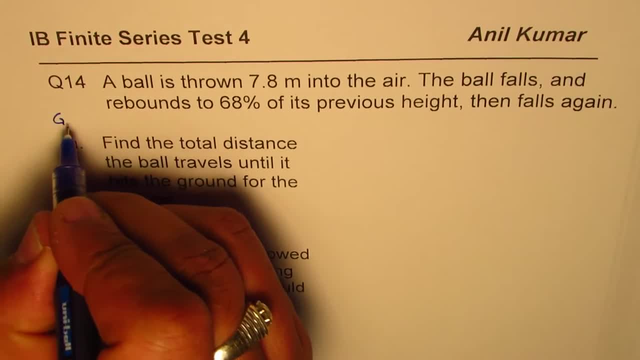 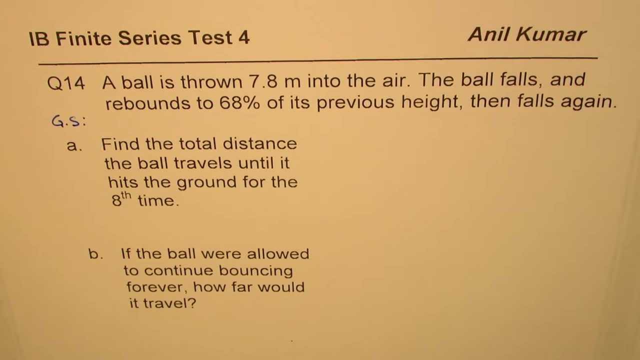 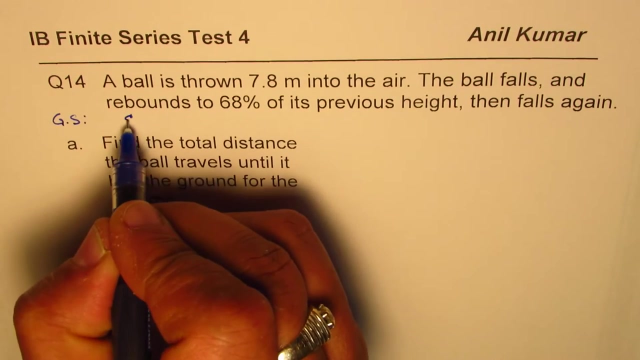 And since it is a geometric series, as you can clearly see here, every time it is 68% of the previous amount, So it is indeed a geometric series. So for a geometric series we have to find total distance and also the distance which it travels when n is infinity. right, So that is. so you need two formulas. So the first formula for the total distance for a geometric series is first term, a times one minus two. 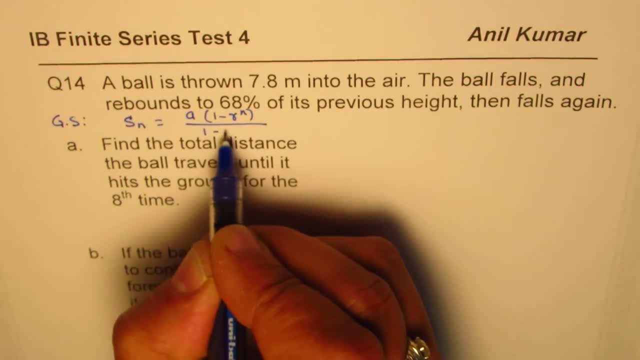 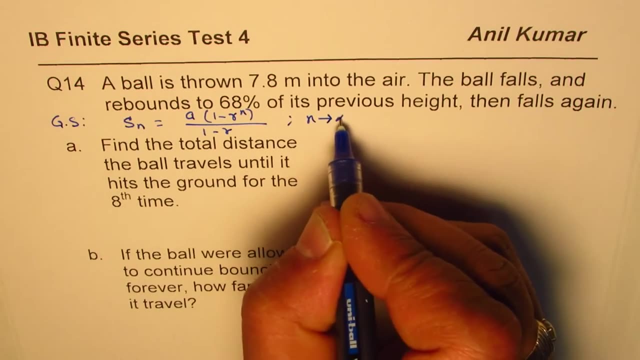 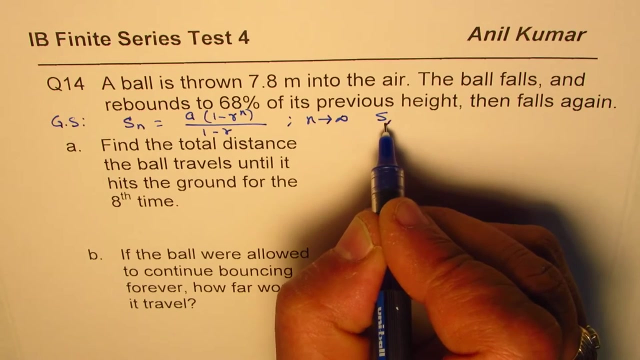 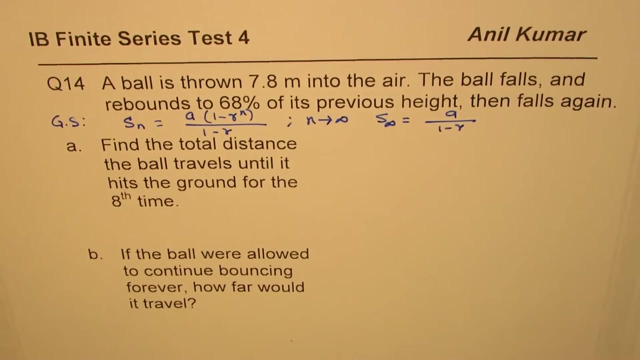 One minus r to the power of n divided by one minus r. And the second when, when n approaches infinity, very large r over n approaches zero. So in that case the sum for infinite number of terms will be equals to a over one minus r. So these are the two formulas for you. You can pause the video, answer the question and then look into my suggestions. 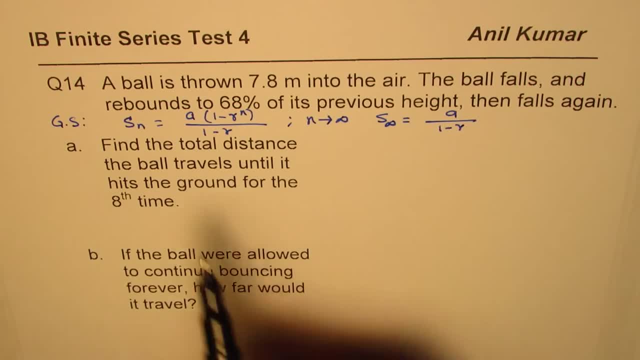 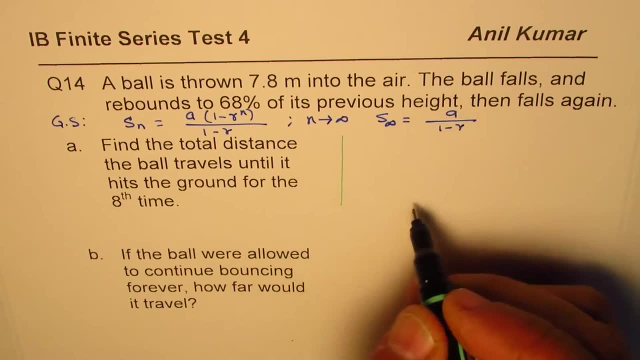 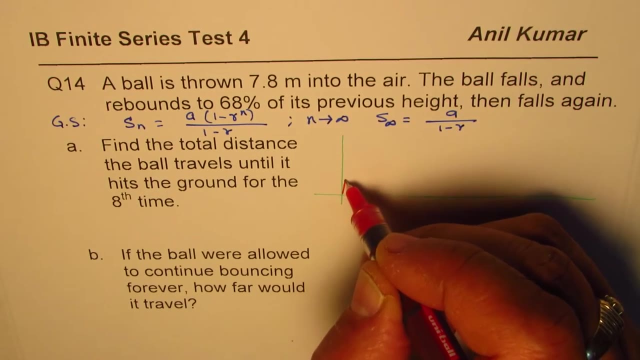 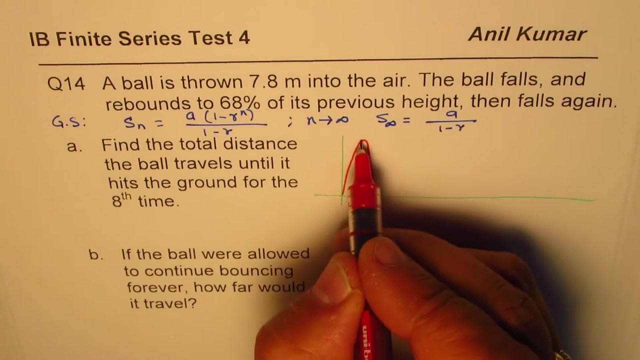 So let's first understand the question itself. A ball is thrown so many meters into the air, So let's assume that the ball is thrown from the ground, Okay so, so we'll just kind of sketch the scenario. So let me just throw the ball like this: goes up and comes down, Okay, so it'll rebound. It goes 7.8 meters. So this height for you is 7.8 meters, Okay. 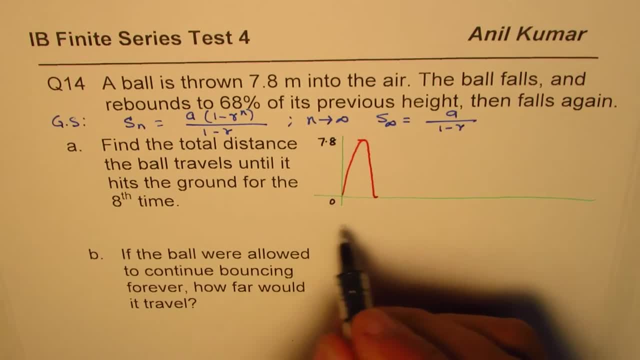 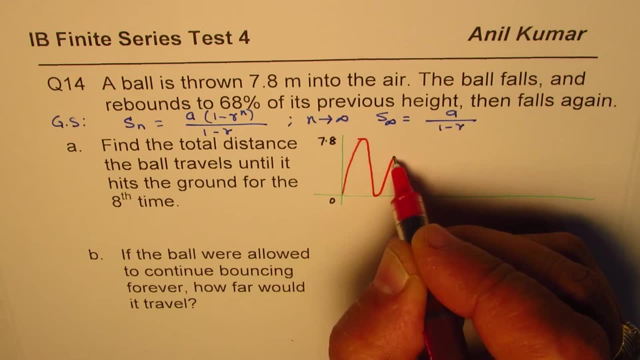 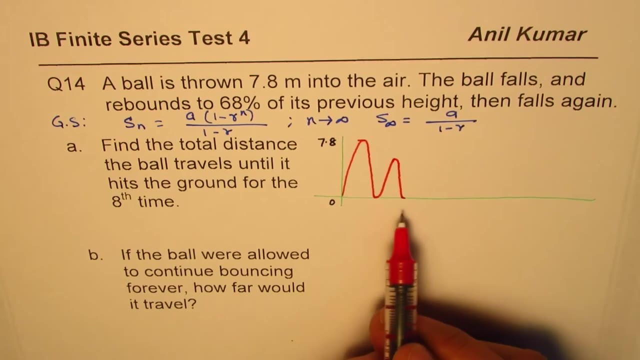 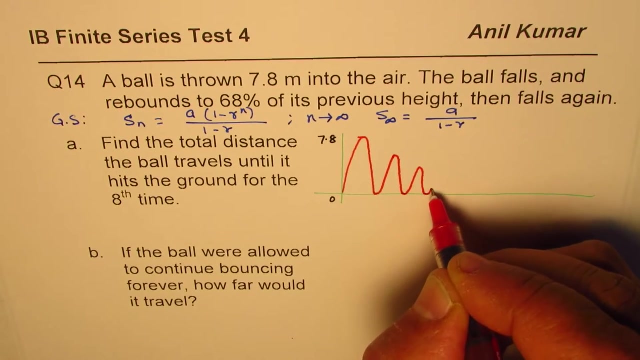 Time t first bounce, right number of bounces. first bounce will be here, right first bounce will be here. then it will go up and only goes up to 68%, slightly more than 50%, and comes down. So that is the second time it hits the ground. So second, and then goes up, and third time goes up, Fourth time goes up. 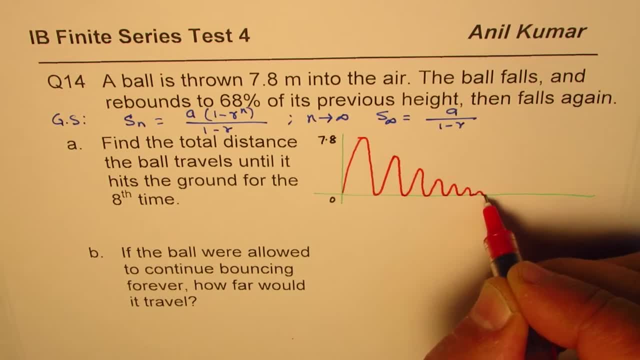 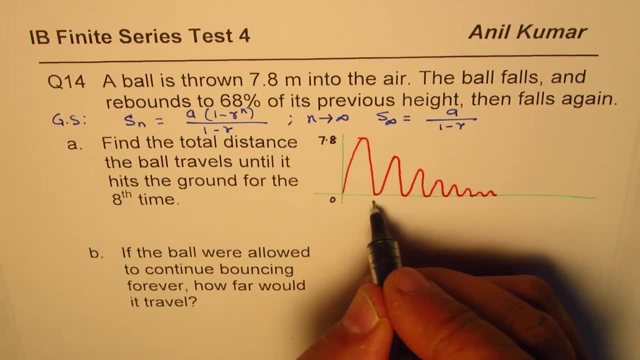 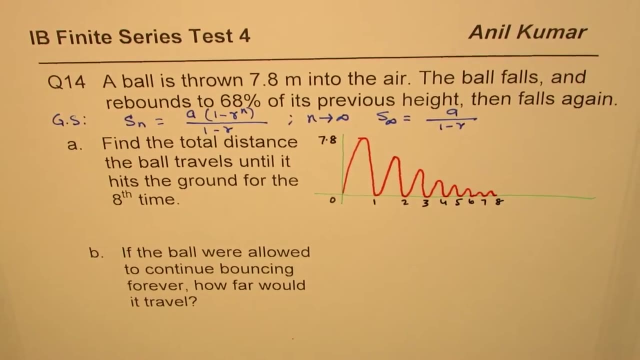 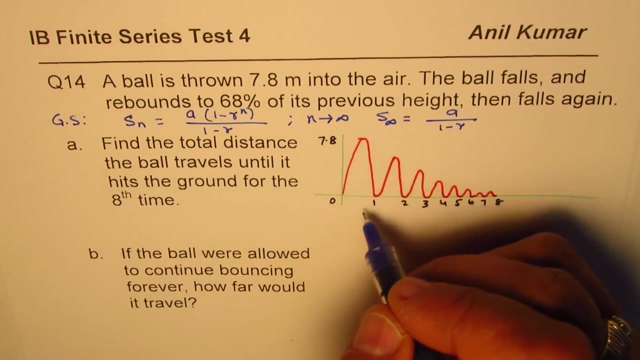 Fifth, sixth, seventh, eighth- Okay, this is kind of bigger Anyway. so eight times, right. So 1, 2, 3, 4, 5, 6, 7, 8.. Okay, so eighth time. So we want total length, which is shown here. This is what we want. You'll observe that it has two types of lengths: One is rising and one is falling, right. 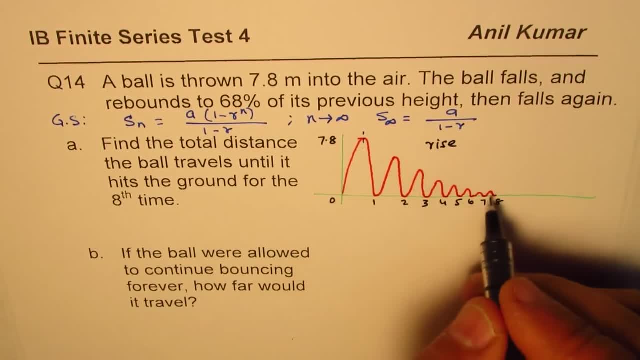 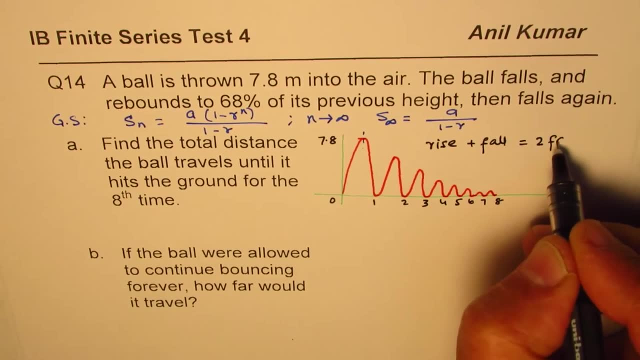 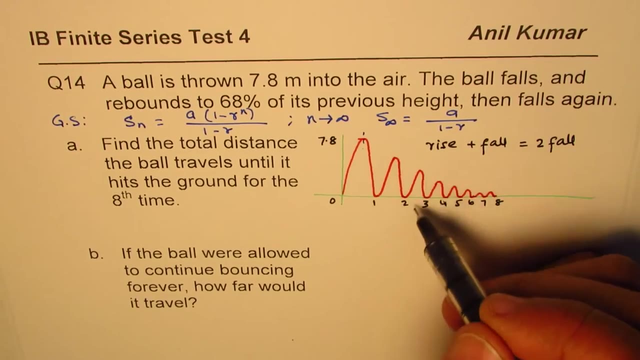 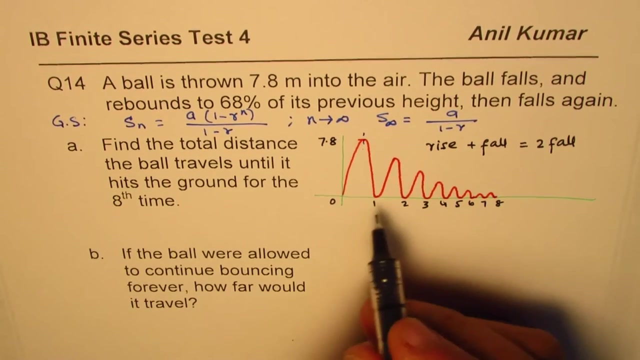 It has two types of lengths, which is rise and then fall, right. Rise plus fall, Now both are equal, So we can say two times fall, Is that okay? So we'll find the length of only falling times, since both are equal, right, So we can actually multiply by two. So s of n, it is kind of geometric series where we are starting with 7.8.. So the series is 7.8.. 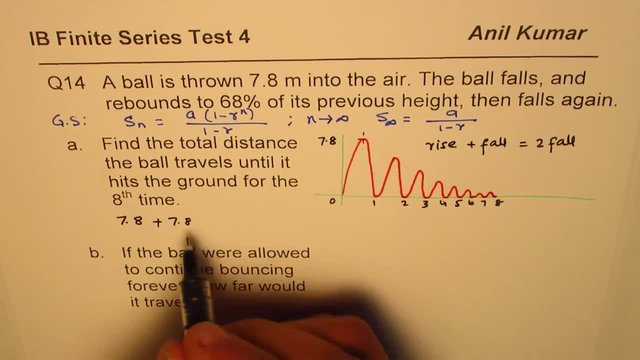 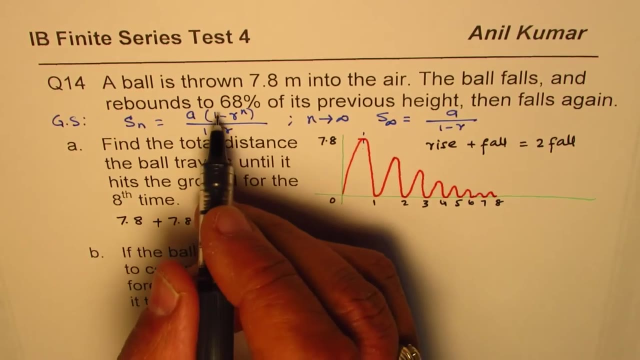 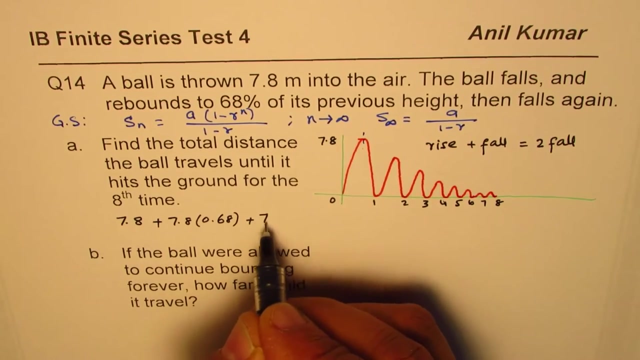 And then we need to add 7.8 times. It goes rebounds back to 68%, right? So r is 68%, right, So. so it is times 0.68,, right 0.668.. And then again it is 7.8 times 0.68 times 0.68.. 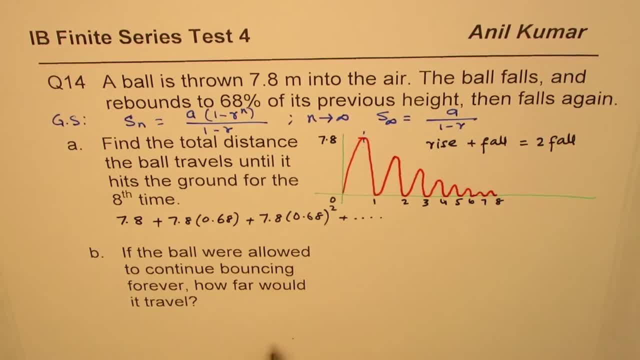 So I'll write this as square and plus so on. Do you see that? And the last term will be- this is the third term- will be 7.8 times 0.68 to the power of 8 minus 1, which is 7, okay. 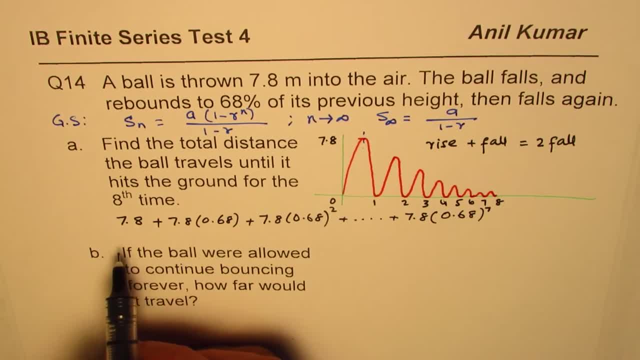 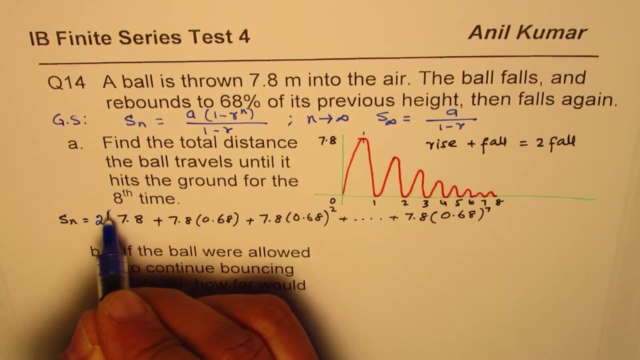 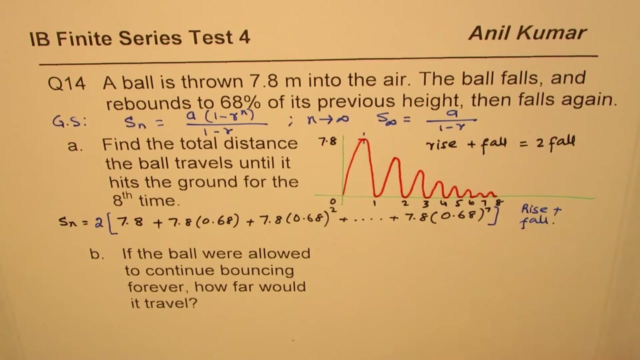 So that becomes your geometric series, right? And we want to find some of this series. So that is s of n, right? This is all falling. What I've done here is we have rising And falling, Is it okay? So we'll multiply this by two To take care of rise plus fall. Do you understand? So that is what we have done. So it's very critical to understand. And then we can always substitute values in the formula and calculate the answer, right. So so our answer will be s of n equals to two times all this, And this is equals to two times. We'll substitute the values. Let me use another ink here. I could have done here. 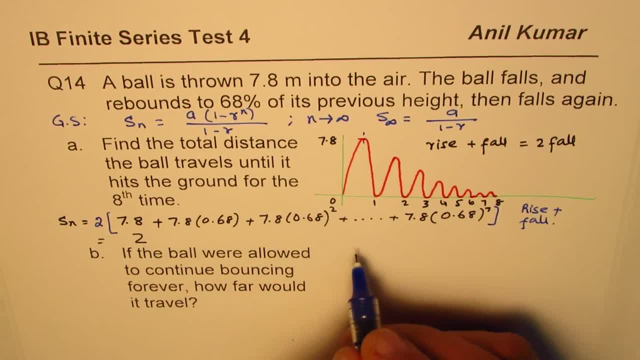 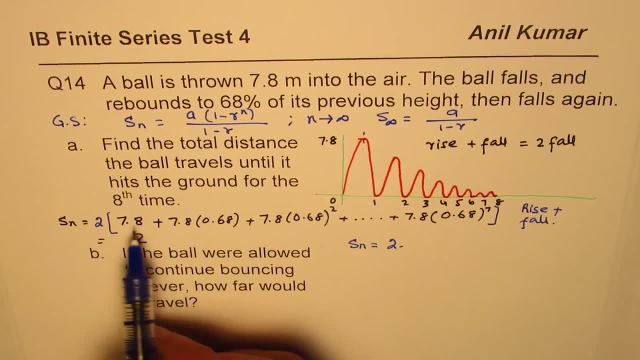 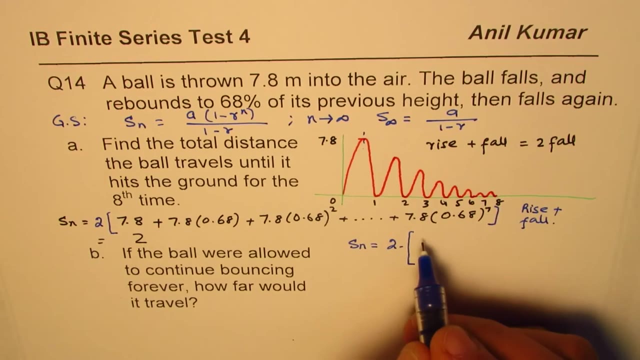 Okay, So let's do it here on this side. So let's do it here. So we have s. n equals to, as I've said here, two times. So two times sum of this series, using the formula First term, is 7.8.. So let me write like this: Okay, that's better. So it is 7.8 times 1 minus r is 0.68 to the power of n. 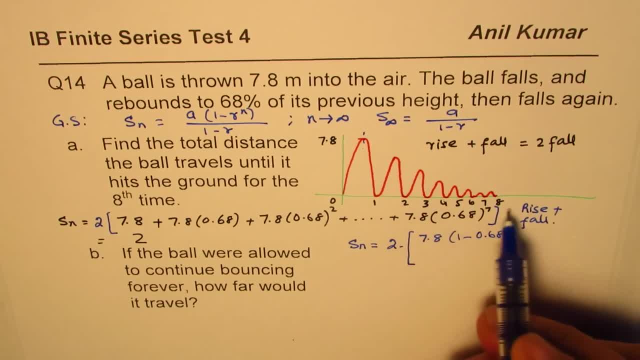 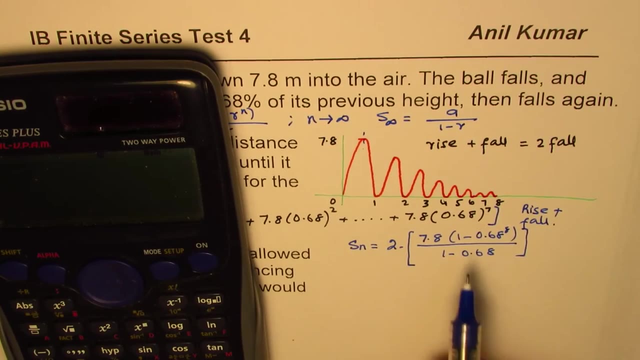 8 times. 8 times is n right? So it goes to the power of n divided by 1 minus 0.68.. Is it okay? So that is what you get. Now let's use the calculator and find the answer right. So what we have here is so we'll do first inside the bracket, then multiply by two. Okay, 7.8 within brackets. 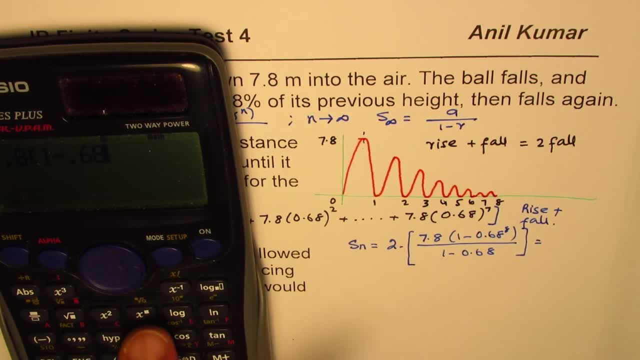 1 minus 0.68 to the power of 8, right Bracket close, And let's say equal to, and then we'll divide by this term right, Divide by within brackets: 1 minus 0.68 bracket close equals to 23.26.. Now multiply by two right, So times two equals two, So it gives us a value which is 46.5.. Let's round it to 46.5.. 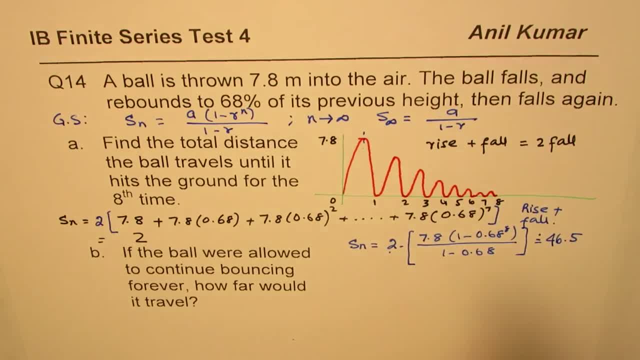 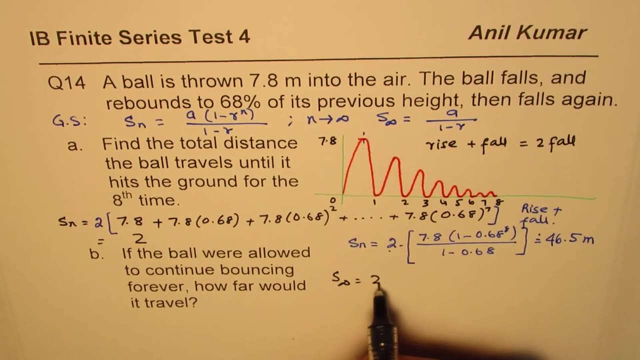 6.5, approximately right, And the units are meters. So that becomes your answer for the part A. right Now let's find the solution for part B. The formula for infinite number of times will be two times Okay, two times A over 1 minus r. That is, two times A is 0.78.. We're talking about falling times right Over 1 minus 0.78. 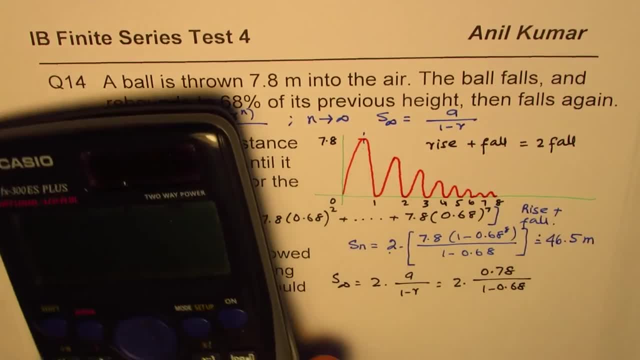 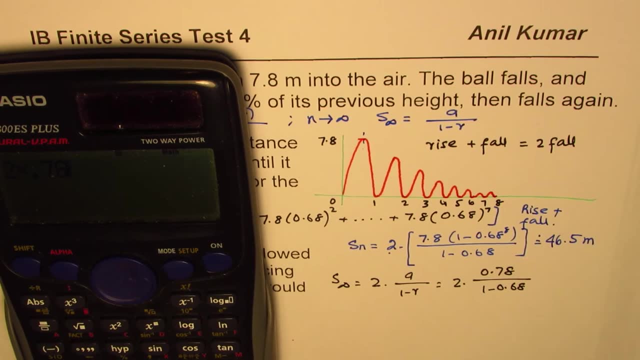 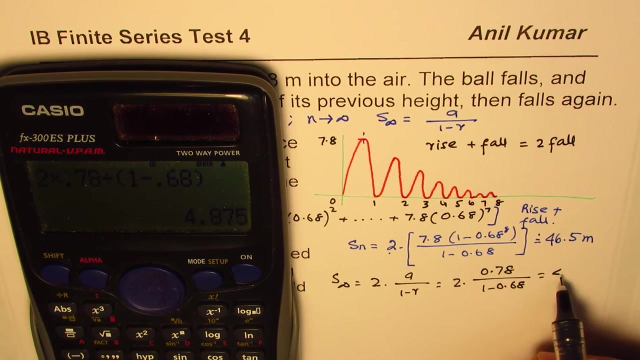 Is it okay? So let's calculate this. So we have two times 0.78 divided by within brackets, 1 minus 0.68- bracket close right Equals to and decimal values for what happened. So something is wrong. Oh, I'm sorry, This is not 0.68..